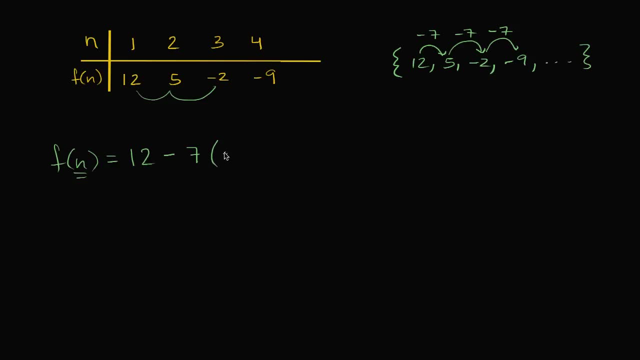 we're subtracting seven, n minus one. we're subtracting seven- whatever term- we're on that term- minus one times. So it's n minus one times And let's see if this actually works out. So f of one is going to be 12 minus seven. 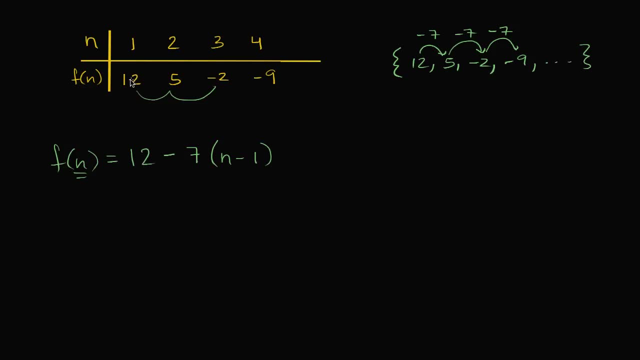 times one minus one, that's zero, So that's all just going to be 12.. F of two is going to be 12 minus seven times two minus one, So it's going to be 12 minus seven times one, or we're just going to subtract seven once. 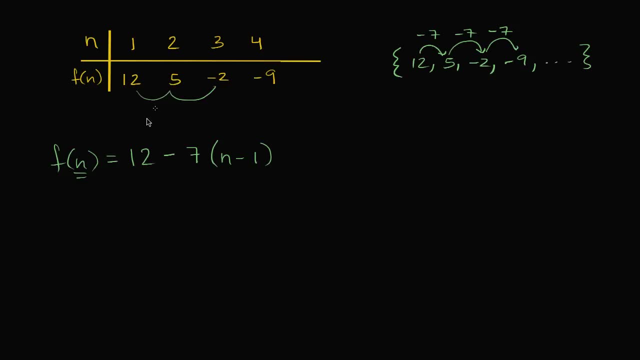 which is exactly the case. We start at 12 and we subtract seven once, F of three. you can keep testing this: 12 minus, and we should have to subtract seven twice And we see three minus one is two times. So we're going to subtract seven two times. 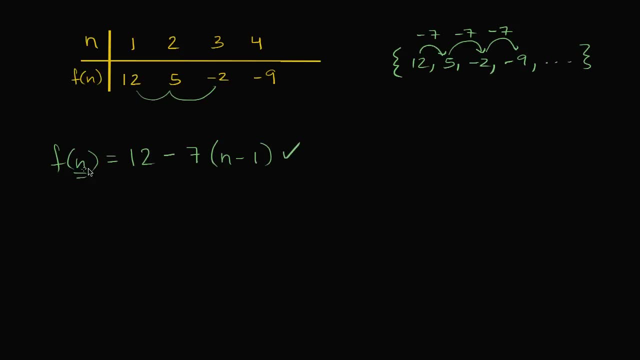 So this looks right on. We've defined the function explicitly. we've defined f explicitly for this sequence. Let's do another example here. So in this case we have some function definitions already here. So you have your sequence. you could kind of view it in this table. 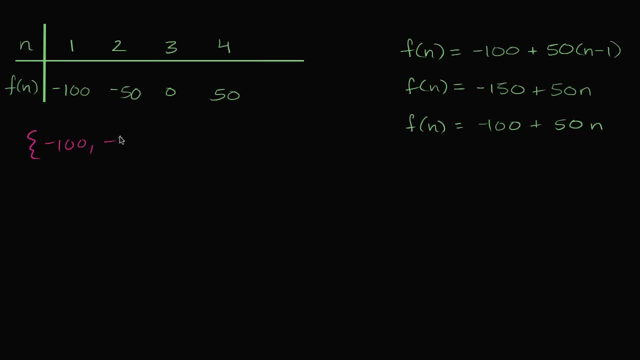 or you could view it as: the first term is negative 100,, next term is negative 50, next term is zero, next term is 50. And it's very clear that this is also an arithmetic sequence. We're starting at negative 100,. 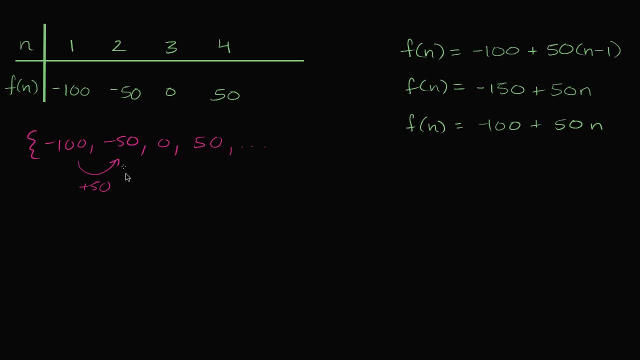 and then what are we doing here? We're adding 50,, and then we're adding 50,, and then we are adding 50,, so each term is 50 more than the term before it, And what I want you to do is pause the video. 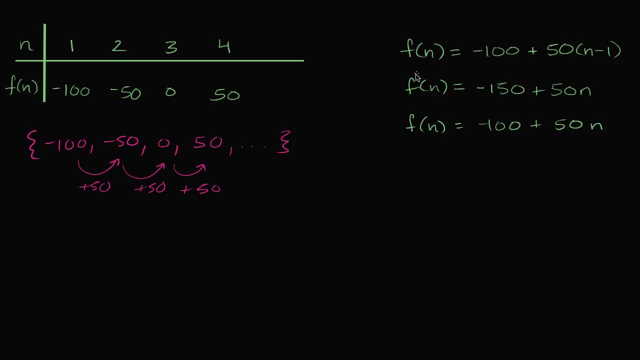 and think about which of these definitions of the function f are correct, and it might be more than one. All right, so let's think about it. So, this definition right over here, one way to think about it, it's saying: okay, I'm gonna start at negative 100,. 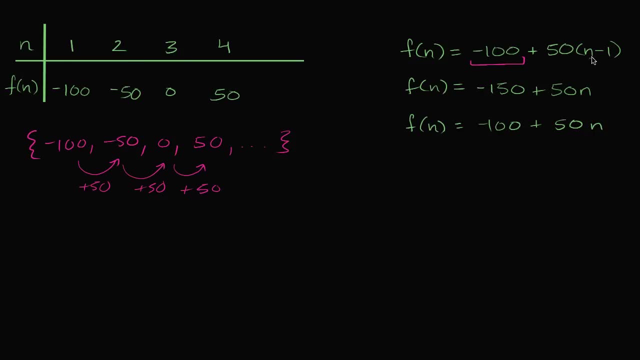 and I'm gonna add 50 n minus one times. Does this make sense? Well, for the first term we're going to if we start at negative 100, we don't wanna add 50 at all. We wanna add 50 zero times, and it works out. 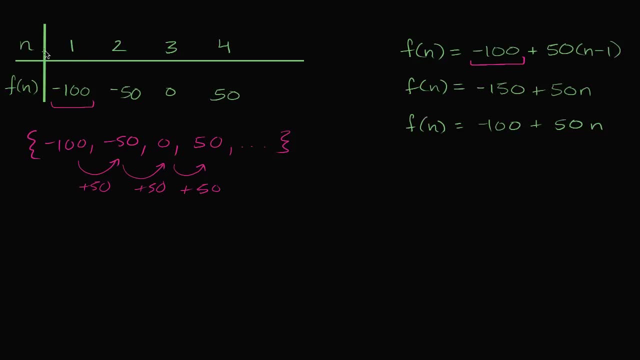 because one minus one is gonna be zero. So it checks out for n equals one. Let's see. for n equals two, you start at negative 100.. I wanna add 50 once. so I wanna add 50 once. It's gonna be a one. two minus one, yep, it's a one. 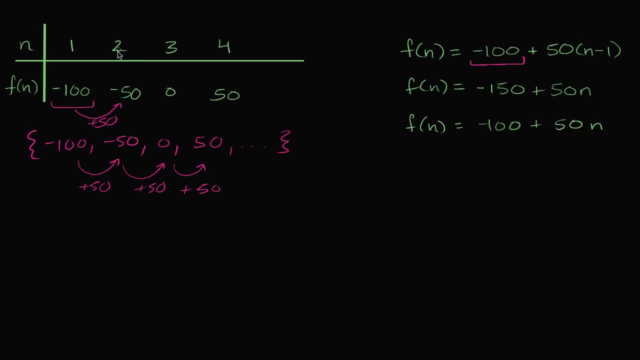 We're adding 50, whatever this number is, whatever n is, we're adding 50, one less that number of times. So for here, we're adding 50 twice. For when n is four, we're adding 50 three times. 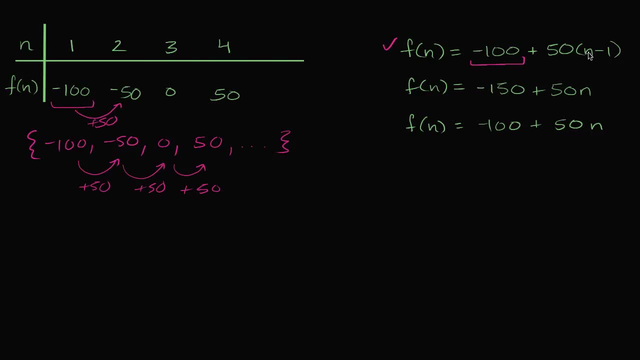 And this one checks out: When n is four, we're adding 50,. four minus one. three times negative. 100 plus 50 times three. We're adding 50 three times. adding 50: one, two, three times. 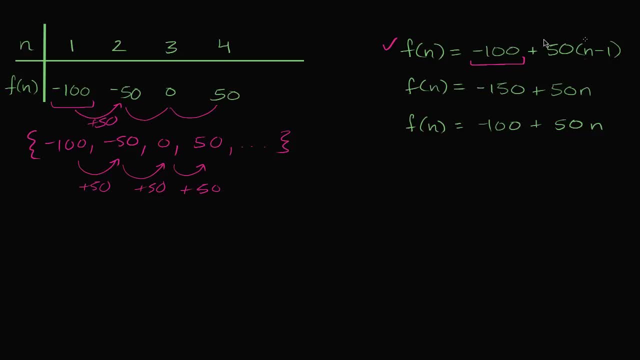 Well, that gives you 50. So I like this one. Now let's see about this one over here. Negative 150 plus 50n. All right, that's one way of saying. so let's see if we n is equal to one. 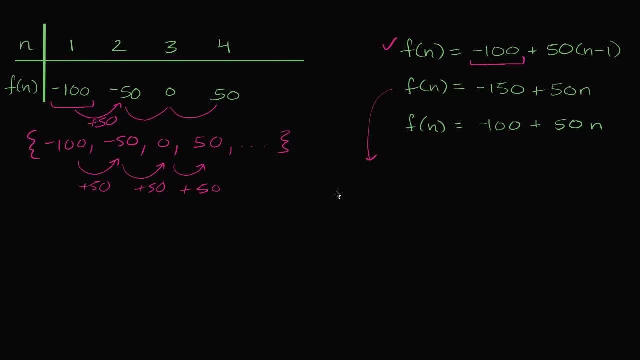 it's gonna be negative. let me actually let me draw a table for this one. So if we have n and we have f of n and this is gonna be for this character right over here, So if n is one, it's gonna be negative: 150 plus 50,. 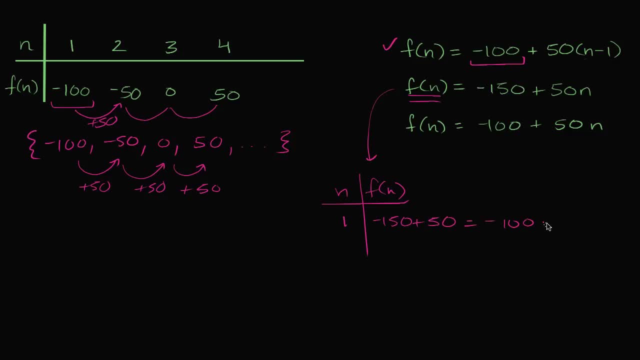 which is negative, 150.. Negative, which is negative 100.. Yep, that checks out. When n is two, we get negative 150, plus 50 times two. 50 times two, which is going to be this is 100, and there's negative 150. 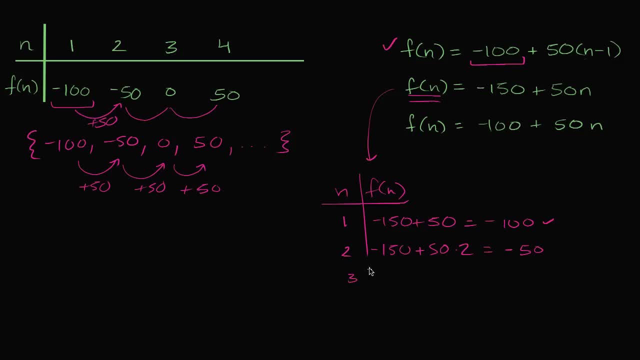 This is gonna be negative 50. When n is three- and that checks out, of course- When n is three, you get negative 150 plus 50 times three, which is equal to zero. This checks out. This one over here is going to work. 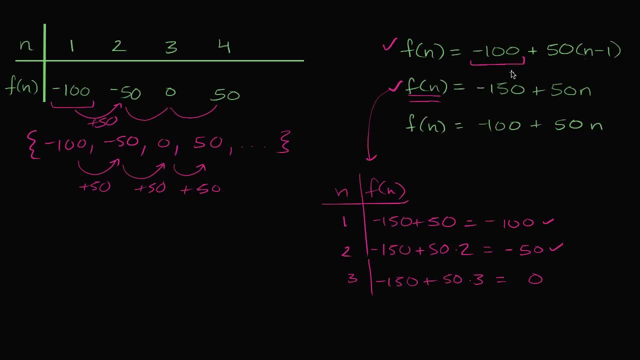 And you might say: well hey, these formulas look different, But you can algebraically manipulate them to see that they are the exact same thing. If you were to take this first one, it's negative 100 plus. let's distribute this 50,. 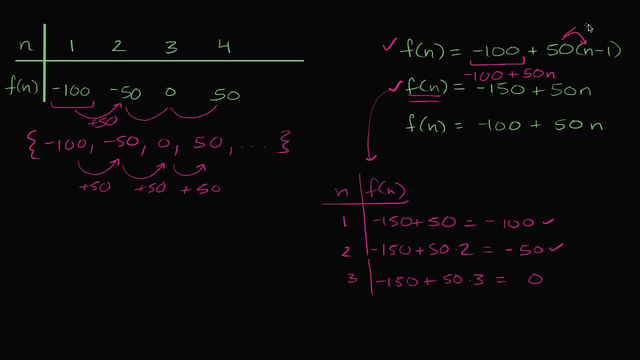 plus 50n, plus 50n, minus 50,, minus 50. Well, negative 100 minus 50,, that's negative 150, and then you have plus 50n. So these are algebraically the exact same definition for our function. 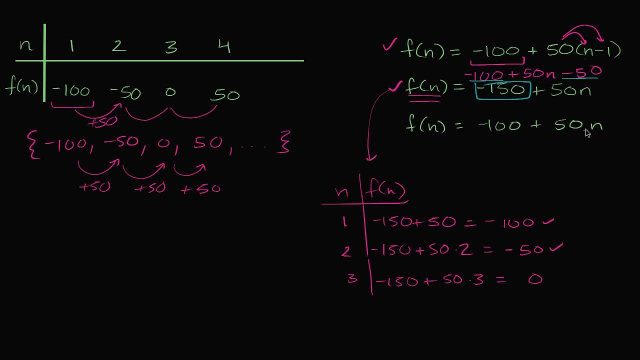 Now, what about this one here? Negative 100 plus 50n. Does this one work? Well, let's see. when n is equal to one, this would be negative 100 plus 50, which is negative 50. Well, no, this doesn't work. 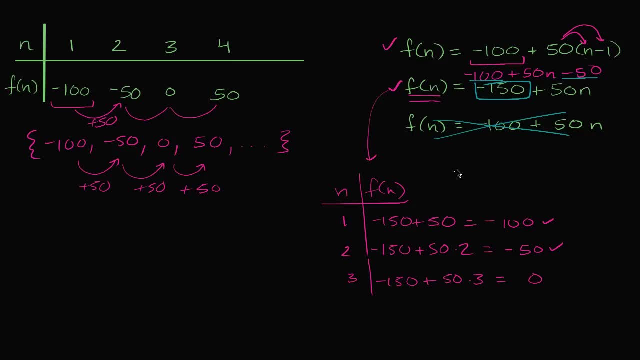 We need to get a negative 100 here, So this one is not not correct. 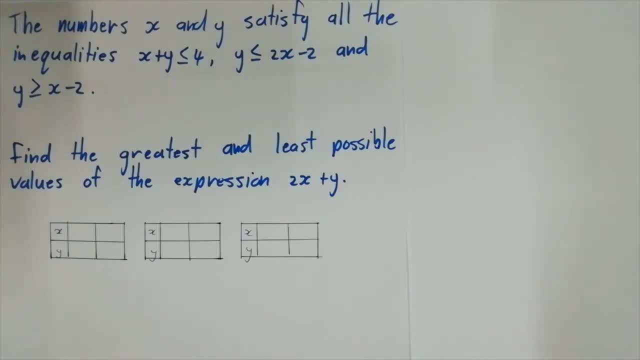 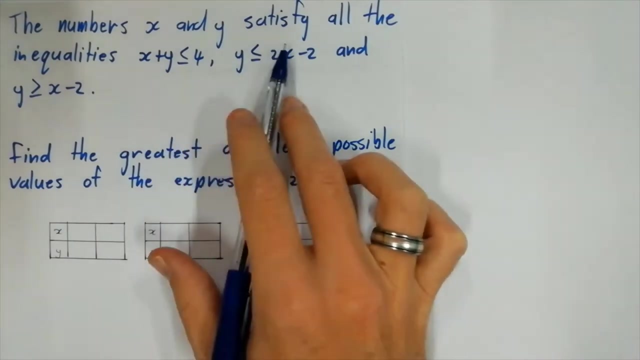 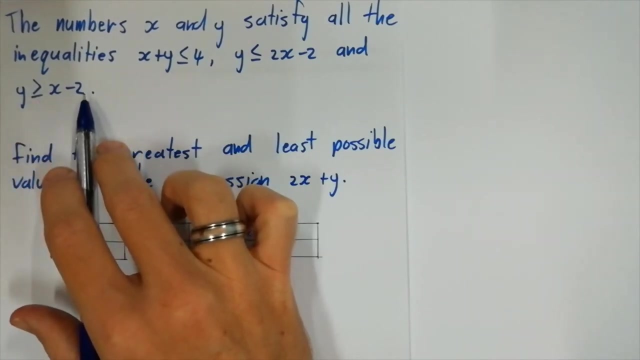 Hello, let's work through this example together. The numbers x and y satisfy all the inequalities. of x plus y is less than or equal to 4, y is less than or equal to 2x minus 2, and y is greater than or equal to x minus 2.. 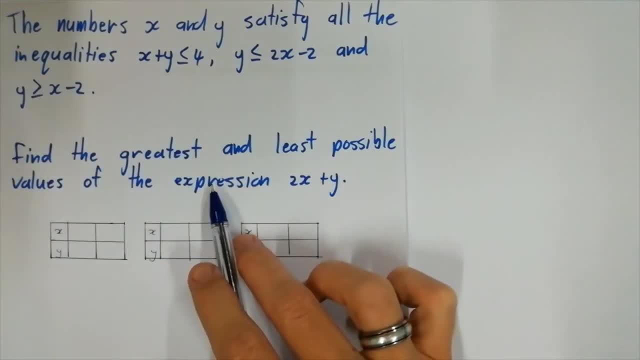 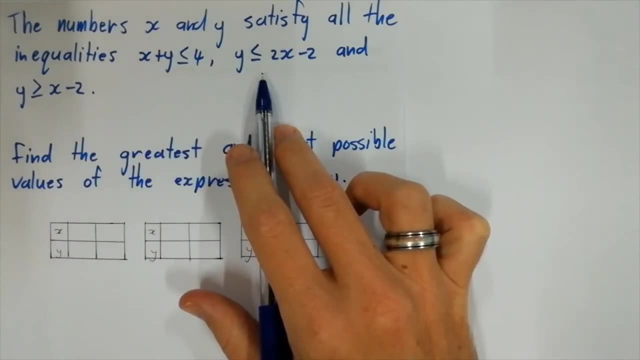 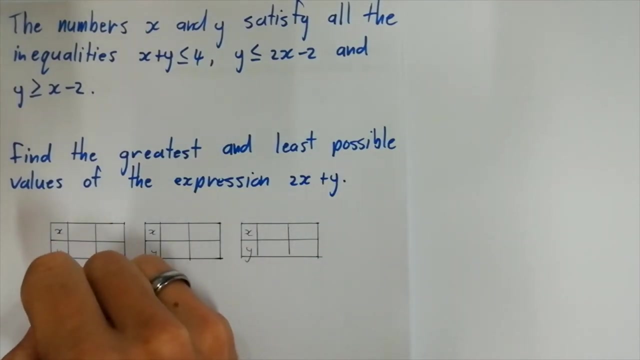 We have a second part to that question. but before we get here let's first sort out these numbers here Let's get some values for them. So for the first one we say: x plus y is less than or equal to 4,. y is less than or equal to minus x plus 4.. 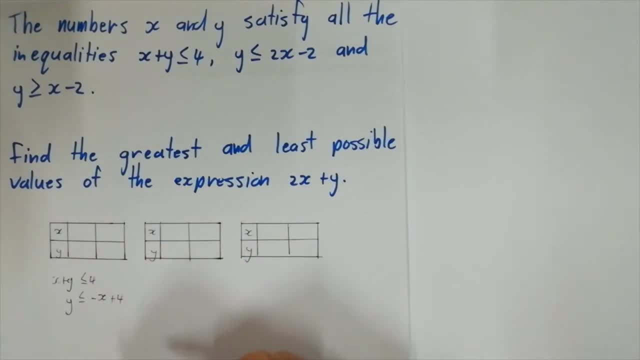 So we can start getting some values in here. We can say: if x is 0,- which is the y-intercept- y would be a positive 4.. If x was 4, that would be a negative. 4 plus 4 would be 0..